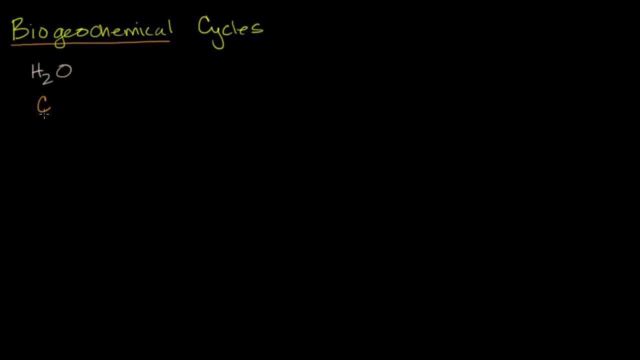 There's carbon dioxide in the air. There's a lot of carbon in organic molecules that form up Most of the mass of life as we know it, And then there's actors that maybe don't get as much attention. There are things like nitrogen. 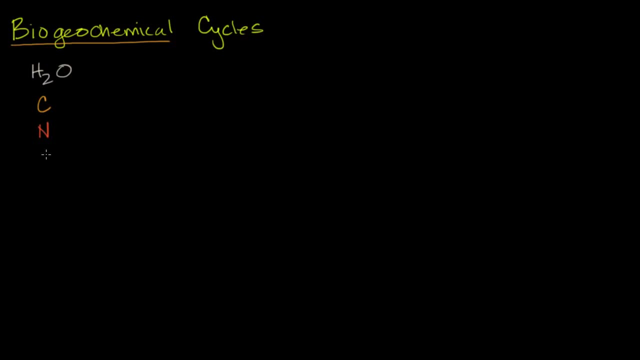 And, of course, you have characters like characters like phosphorus, And you might say, okay, I get that. most organic molecules are made up of a bunch of carbons and hydrogens and, every now and then, oxygens. but what about nitrogens and what about phosphorus? 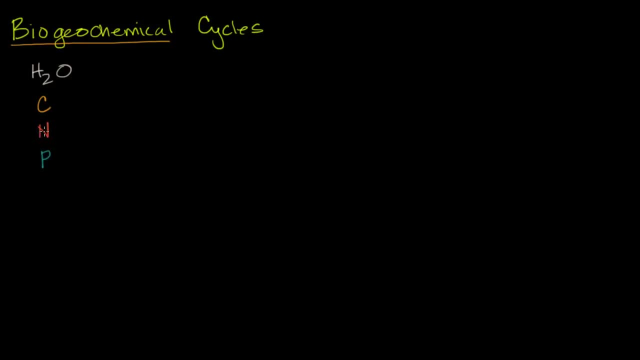 And remember your DNA, deoxyribonucleic acid. we're talking about nitrogenous bases, Your adenines and guanines and all of these things that we talk about in DNA. they involve nitrogen. And there's other biomolecules, amino acids, proteins. 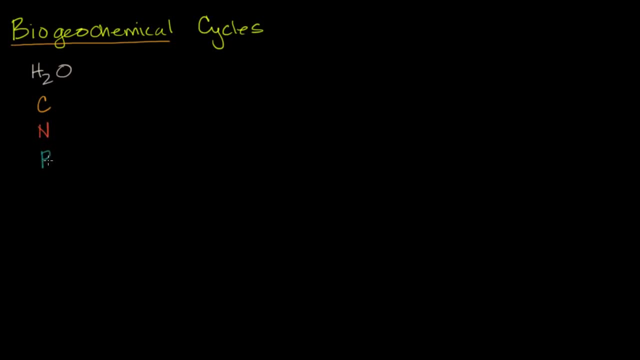 amino acids, which make up proteins that involve nitrogen, Phosphorus, ATP, the identicine triphosphate. It's essential in that core biomolecule. It's also in the backbone of DNA. So these are all essential elements for life And the key thing is is that they all get recycled. 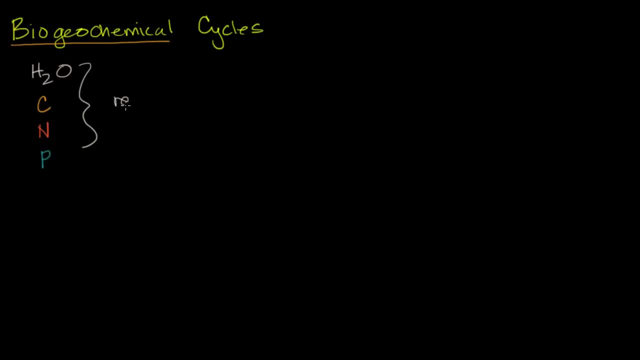 through biogeochemical cycles, So they are all recycled. We talked about how an ecosystem energy flows. It might start with light energy from the sun and then over time, as it's transferred from one form to another, as it flows from one form to another. 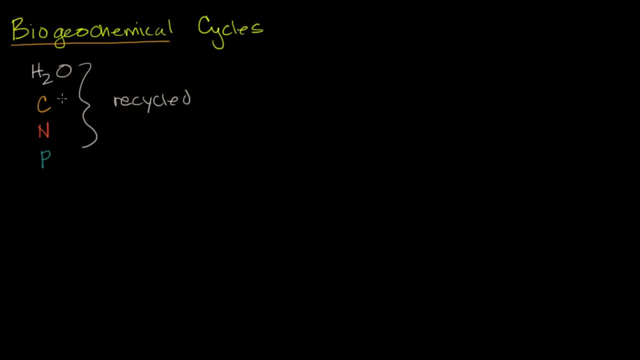 it gets dissipated as heat. But the matter, the elements, the molecules here this is recycled, It was originally formed. I mean, there's a few meteorites that hit every now and then, But the most part, most of the matter. 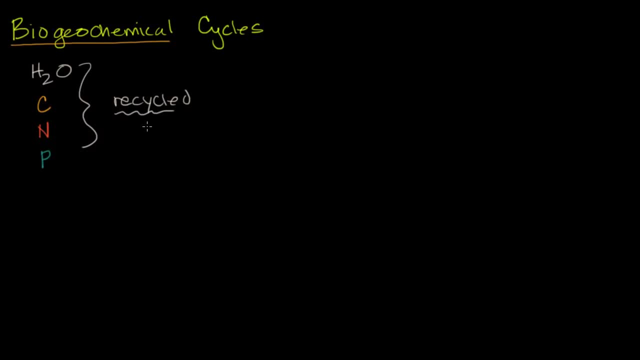 the matter around us was here at the dawn of when the Earth was first formed. It was first created in the inside due to fusion reactions of stars billions and billions and billions of years ago. So all of life, everything that we've seen so far. 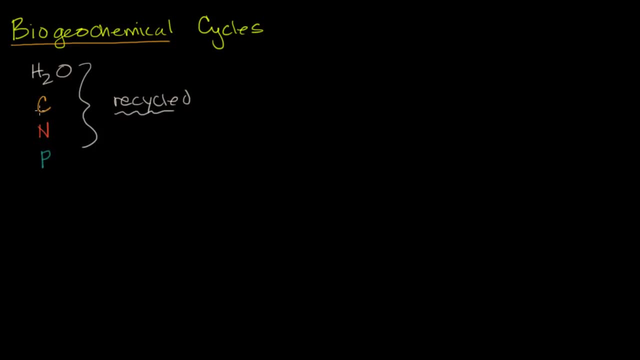 in the history of Earth, for the most part is just the same elements and the same molecules that have been recycled over and, over and over again, And so when we think about biogeochemical cycles, we will think about things like, if we're talking about H2O. 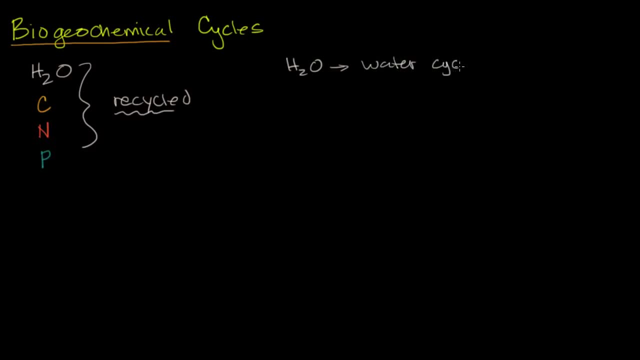 we're gonna think about the water cycle. Water cycle And we have a whole video on that, but just the short version of it is: you could have water actually stored in multiple different ways. Some of it can evaporate as water vapor. Eventually it condenses in the form of clouds. 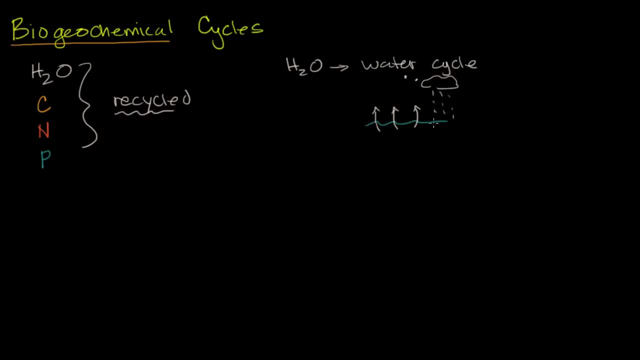 and then it can rain back down And along the way you can have animals. animals get access, especially to the fresh water and make that part of the actual living organisms. You actually also have living organisms that view the water as part of their ecosystem. 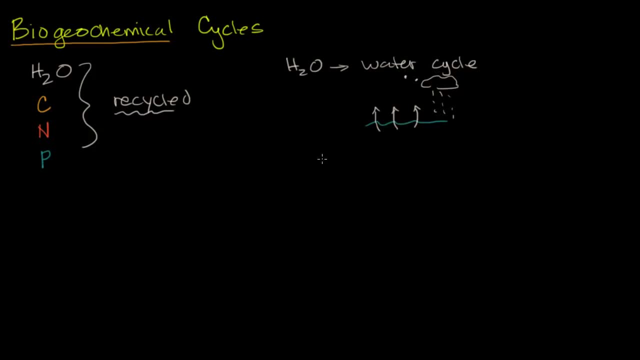 but we go into some depth in another video You'll also hear people talk about, if we're talking about carbon, the carbon cycle, The carbon cycle And just as a very high level overview of the carbon cycle. so let's say that's the ground. 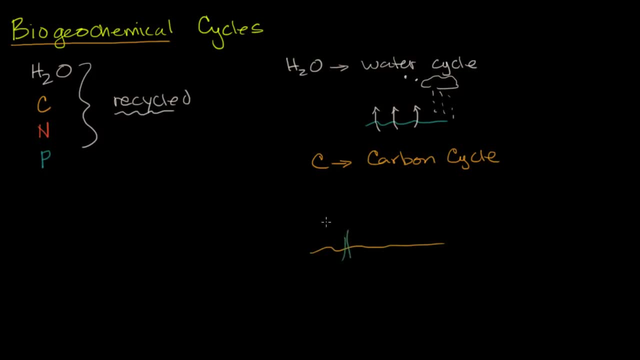 Let's say that this is a plant right over here. It's a primary producer, an autotroph. We talk about that in our ecosystem videos. Let me draw a leaf here. This is a plant that is growing What it's doing while it takes light energy. 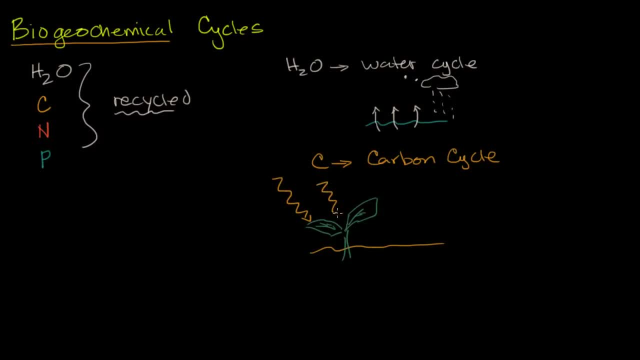 so it gets light energy from the sun. so that's the light energy right over there and it uses that light energy to fix carbon, The carbon that is making up this plant. it's just not emerging out of nowhere. It's being recycled. 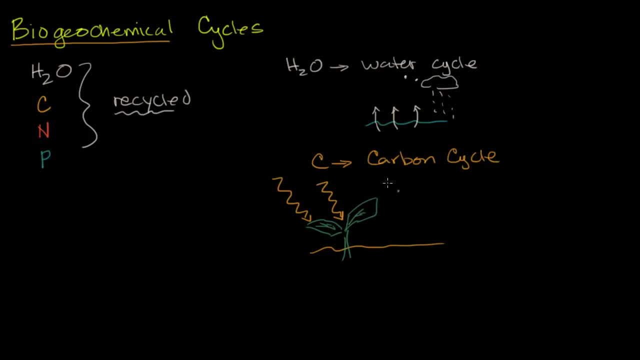 It's being recycled from carbon molecules that are in the air. So the carbon molecules in the air they're going to be, or the carbon in the air it's going to be in molecular form. in terms it's going to be carbon dioxide. 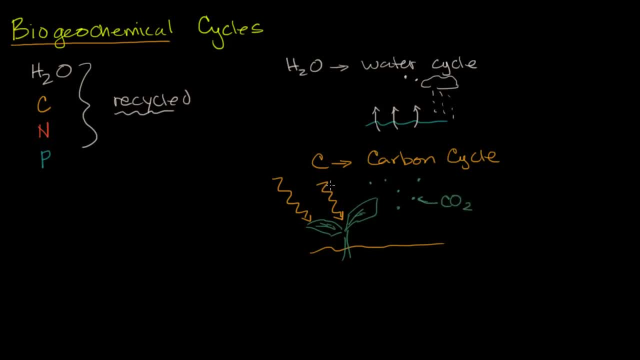 So that over there is CO2. And so the plant uses that light energy and that CO2 gas and it's able to fix the carbon to construct it. So it looks like that plant is just growing. It's not clear where all that mass is coming from. 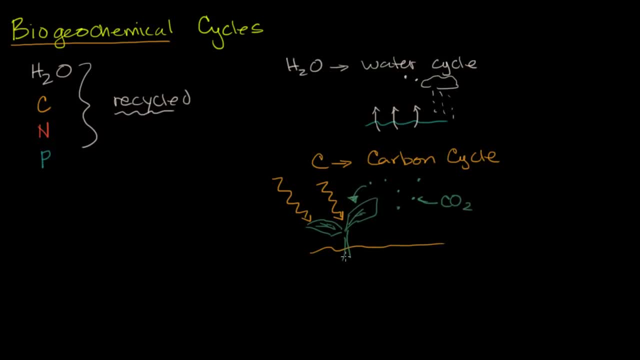 but it literally is coming from the air And it might be able to get. it might get a few of the nutrients, especially things like that like nitrogen and phosphorus, from the ground, And that's where we could go into the whole. 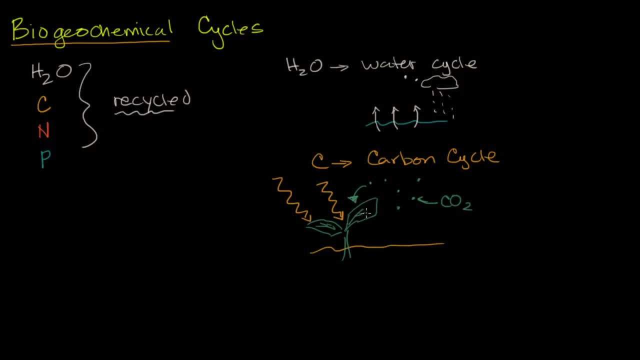 nitrogen and phosphorus cycles, But then, once these plants fix all of this carbon, some of it it gets stored in the biomass. Sometimes the plant dies and then it gets buried and then, with enough pressure, it can turn into hydrocarbons. 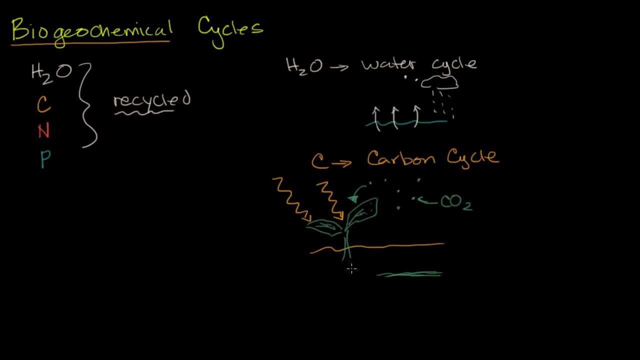 So hydrocarbons when you fuel your car, it's really energy stored by dead plants. a long, long time ago that got buried and put into that form, But it was essentially plants, through photosynthesis, that first stored that energy. But then, of course- and we've talked about this- 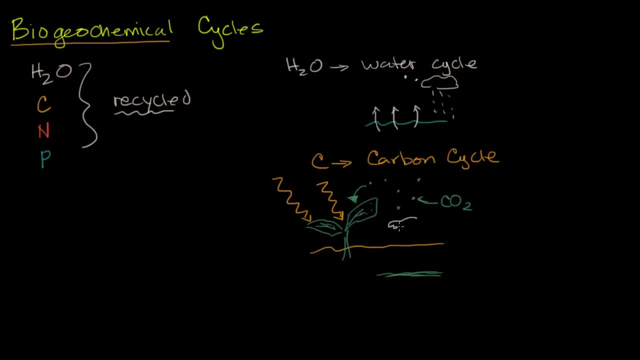 you can have animals that eat those plants. So let me draw an animal that is eating it. So that looks like an animal. Well, that one looks like something that likes to eat more than just plants. So this is. let me draw it like it's like. 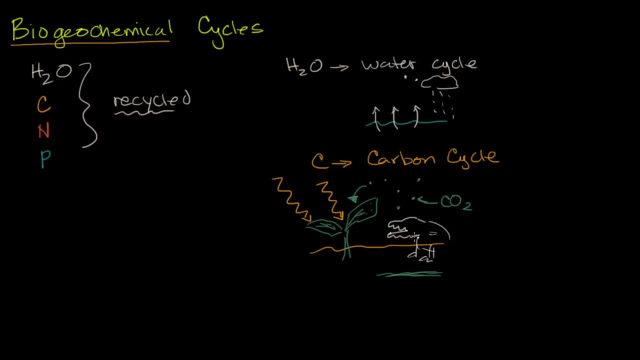 an alligator, chicken-looking thing. Well, that's close enough. Well, you get the idea. When it eats that plant, it's using some of that carbon that was fixed originally by that plant for its own biomass, but it'll also, as it metabolizes, the some of it. 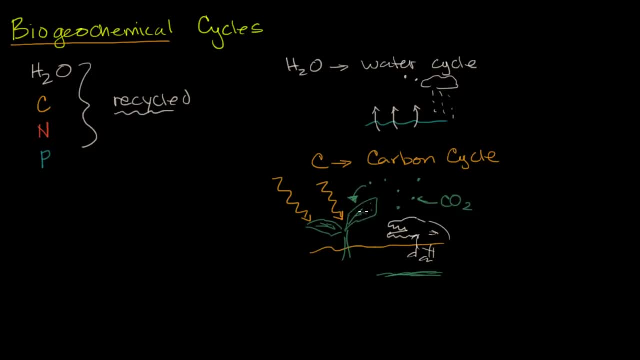 it will use that the bond, the energy stored in those chemical bonds, to live and grow and move about And as it does that, it will exhale the CO2 so that the CO2 goes back into the environment, And this is a huge oversimplification of the carbon cycle. 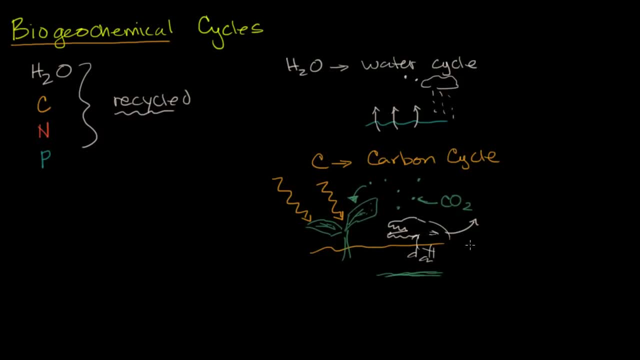 but this is the general idea, And eventually this thing might die or might get eaten by other consumers. And then you have the decomposers down here who could further make use of those chemical bonds that the primary producer first created using that light energy. 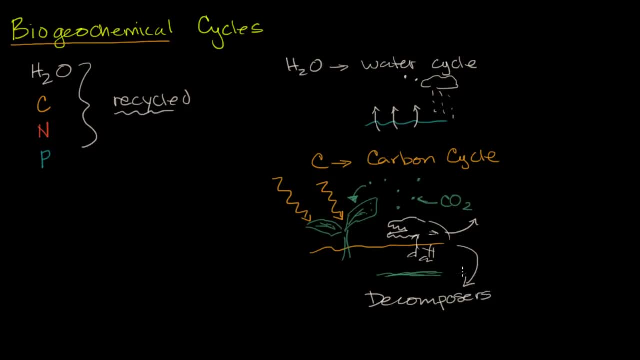 Let me decomposers right over here, And they might also, as they consume that, release more CO2, which will eventually then get fixed again by a primary producer. And there's similar cycles for nitrogen and phosphorus, These often involving bacteria to fix the nitrogen. 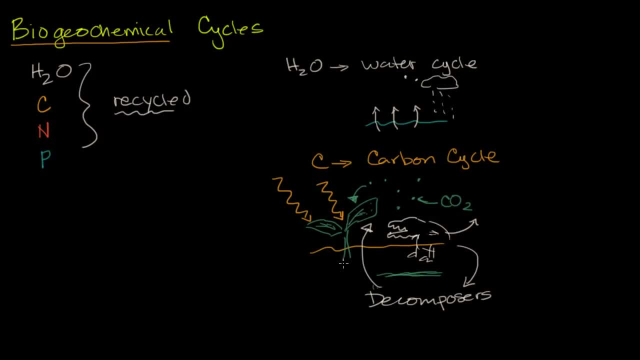 and the phosphorus from the air to make it available as nutrients in the soil. for some of the primary producers in, say, the carbon cycle And nitrogen doesn't get a lot of attention, but this is actually the most common gas in our atmosphere.